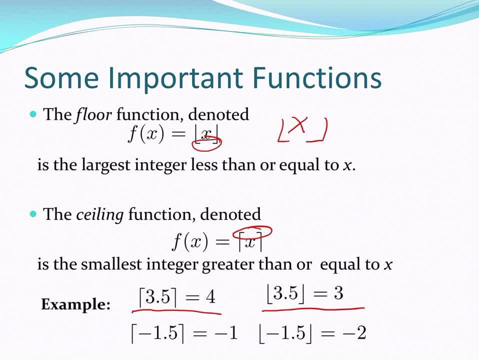 Note that the negatives. we have to be a little bit careful. the ceiling of negative 1.5 is negative 1, because negative 1 is greater than negative 1.5 and the floor of negative 1.5 is negative 1.5.. 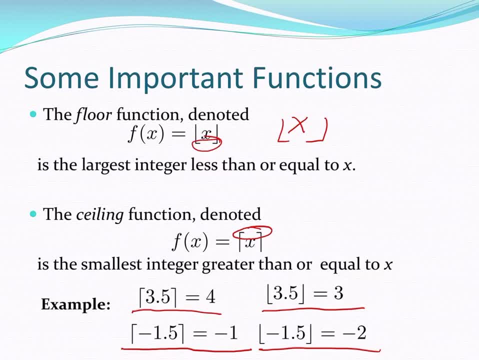 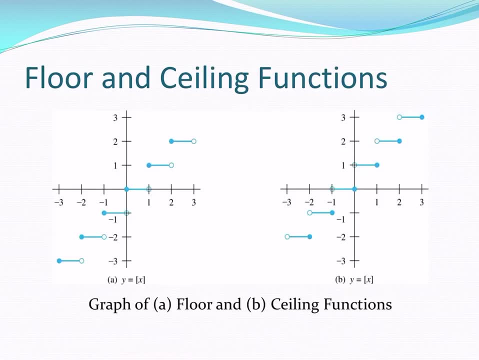 So the ceiling function of 3.5 is going to be negative 2, since it is less than negative 1.5.. Okay, this slide. we have a graph of it. small error here. so this is the four functions. this is going to be x, floor function. this is the ceiling function. so this will be x ceiling function. 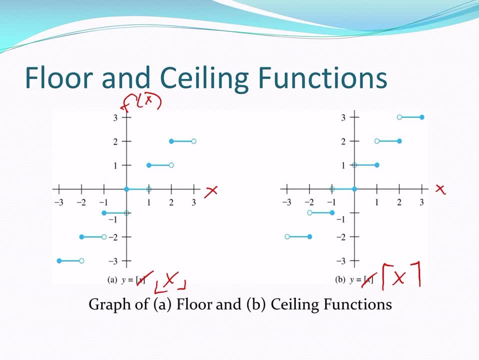 so here's x, here's f of x and we're going to get x, and whenever x is between 0 and 1, not inclusive of 1, we return 0. whenever x is between 1 and 2, not inclusive of 2, we get 1, and so forth. so these graphs look the. 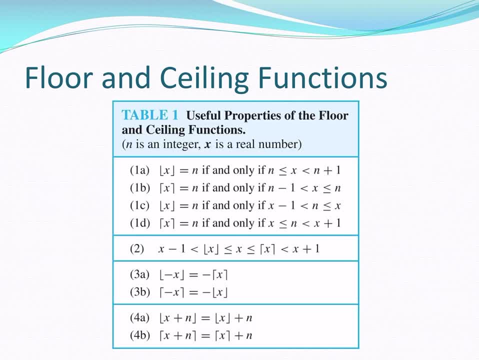 same, except they're shifted up in the case of the ceiling function. Now let's look at the properties of the ceiling functions and floor functions. The floor function of x, a real number, is equal to n if, and only if, n. x is between n and n plus 1, inclusive of x of n. 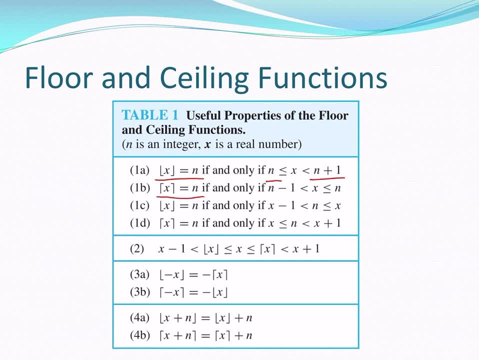 and the ceiling function of x is equal to n, if, and only if, x is between n minus 1 and n. x in plus 1, inclusive n. you can derive these next two from the first two, where the floor function of x is equal to n, if, and only if, x minus n is between x minus 1 and. 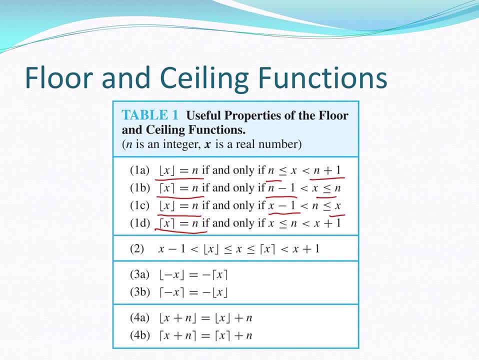 x, inclusive of x, and the ceiling function of x is equal to n if, and only if, n is between x and x plus 1, inclusive of x, Notably that x minus 1 is strictly less than And the floor function which is less than or equal to x, which is less than or equal to the ceiling function, is strictly less than x plus 1.. 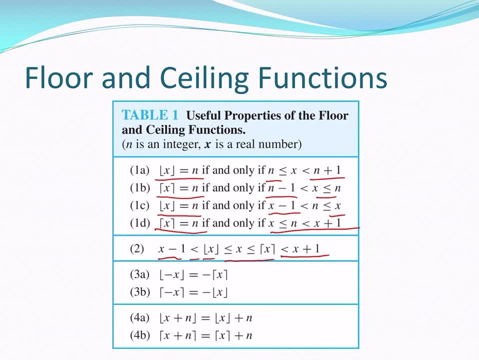 Note that the floor function of the negative is equal to the negative of the ceiling function And the ceiling function of the negative is equal to the negative of the floor function. You could look at our power example with negative 1.5 to illustrate that. 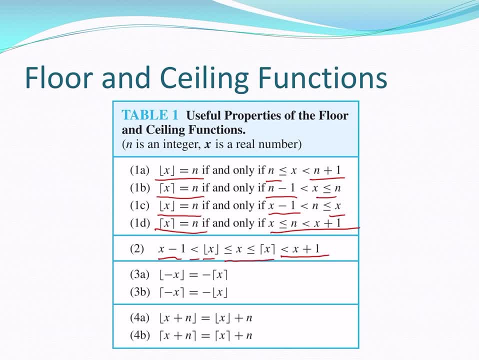 And finally, the floor function of x plus an integer is equal to the quantity, is equal to the floor function of x plus the integer, And the floor function of the ceiling function of x plus an integer is equal to the ceiling function of x plus that same integer. 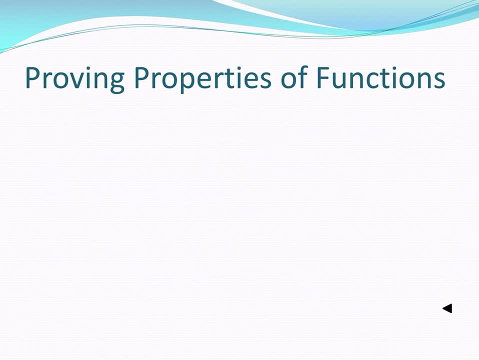 We're going to do a proof of a proposition using floor functions. Here I have 2x. the floor function of 2x is equal to x plus the floor function of x plus the floor function of x plus 1.5.. So say that again. 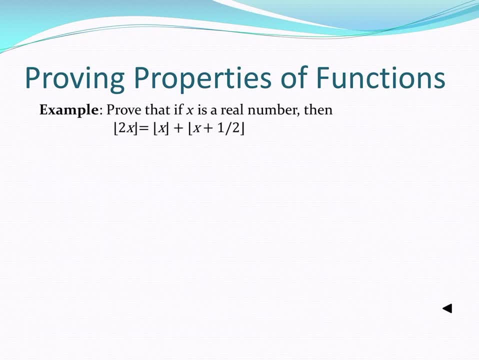 The floor function of 2x is equal to the floor function of x plus the floor function of x plus 1.5.. Alright, we'll do it in two cases. First, we'll say that x is equal to n plus epsilon, where n is an integer and epsilon is a. 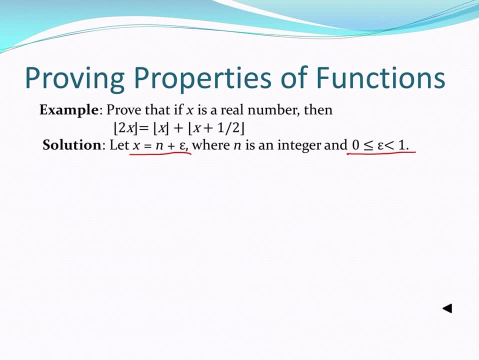 real fraction between 0 and 1, inclusive of 0. So when epsilon is 0, then x is equal to n And we'll have two cases: One where epsilon is strictly less than 1.5.. And the nice thing about this assumption is that twice epsilon will be strictly less than 1.. 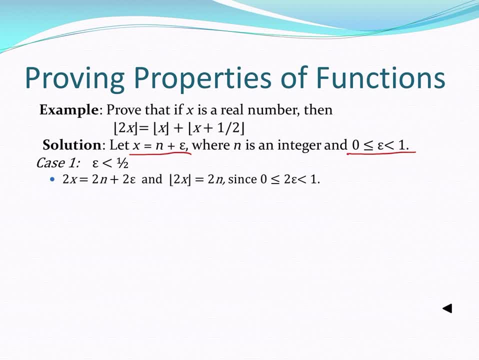 First, let's take a look at the 2x portion of our equation, Since 2x, Since 2x is equal to 2n plus 2 epsilon, and I just mentioned that 2 epsilon will be strictly less than 1,. 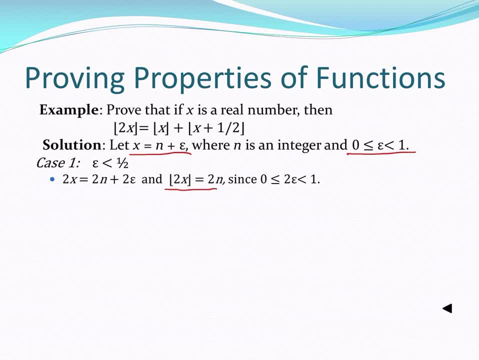 then the floor function of 2x will equal to 2n. Alright, and since the floor function of x plus 1.5 will also equal to n, because since epsilon is strictly less than 1.5, and epsilon plus 1.5 is strictly less than 1,. 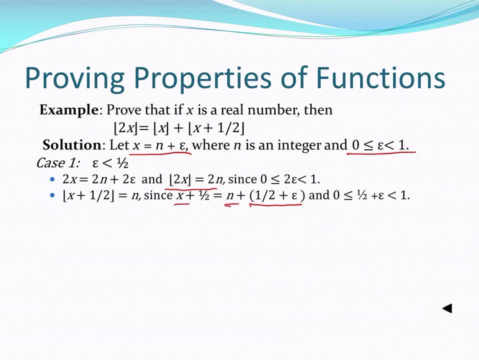 and so the floor function of x will equal x plus 1.5 will equal 2n. And now we can combine them all together. We already know that the floor function of x is equal to n. So, since the floor function of 2x is 2n and the floor function of x plus 1.5 is equal to n plus n, 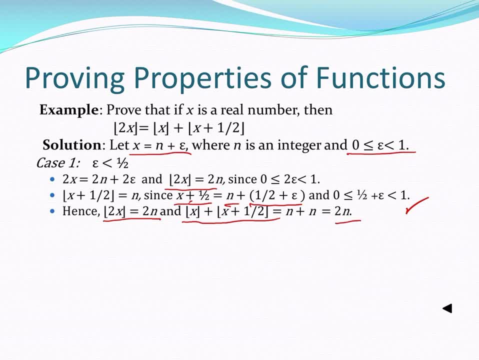 which is 2n. it works for the first case. Now let's take the remainder of the second case, which will be epsilon greater than or equal to 1.5.. Remember, it'll still be strictly less than 1.. 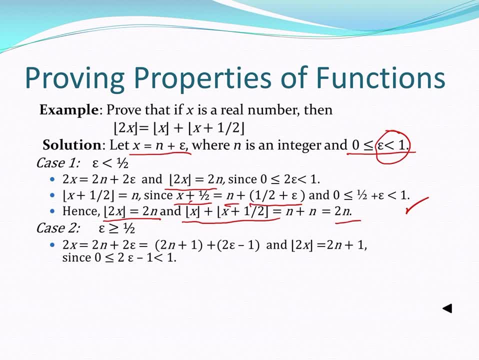 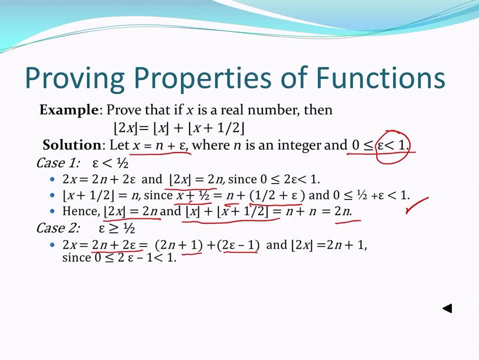 So since epsilon is greater than or equal to 1.5, then 2 epsilon minus 1 will be between 0 and 1.. And so the floor function of 2x will be 2n plus 1.. And now let's take a look at x plus 1.5. 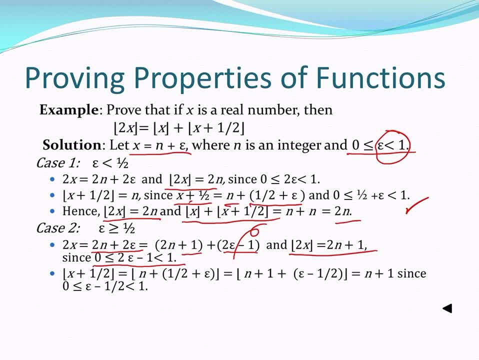 Since x plus 1.5 is equal to n plus 1.5 plus epsilon, I can add and subtract a half, So I'll get n plus 1 plus epsilon minus a half, And we know that epsilon minus a half will be between 0 and 1.. 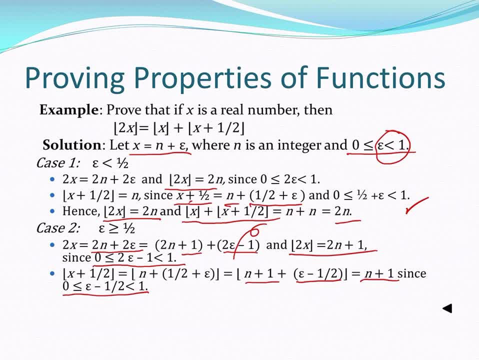 So the floor function of x plus 1.5 will equal 2n plus 1.. And I'll combine those all to get 2x is 2n plus 1.. The floor function of x plus the floor function of x plus 1.5 is n plus n plus 1.. 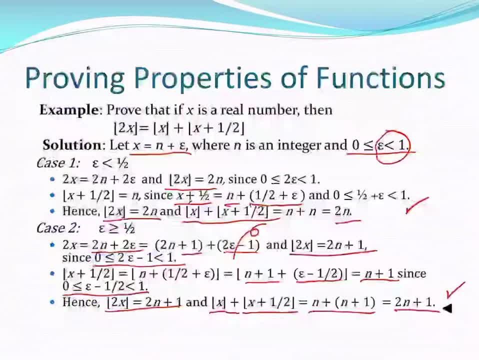 Which is also 2n plus 1.. And we've proven it for the second and all of the cases. So this proposition is proven.